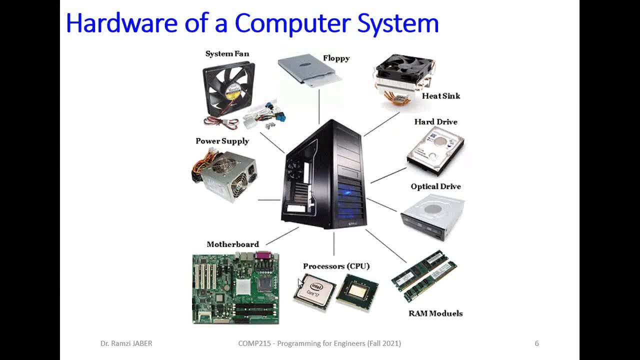 board then we put the cpu the processor inside it then we put here the ram in memory then we put on external pci slots here external sound card or modem or vga here and so on and so on and so on and we have optical drive cd-rom dvd-rom blu-ray and others also we have normal hard disk and today we have ssd hard disk or we have nv mea hard disk also above the cpu because the cpu will be very hot very very hot so we put above the cpu the heat sink with the fan aluminum plus fans okay to cool down the cpu on all the computers was using floppy disk today we don't have floppy disk we have alternative like flash memory usb flash memory 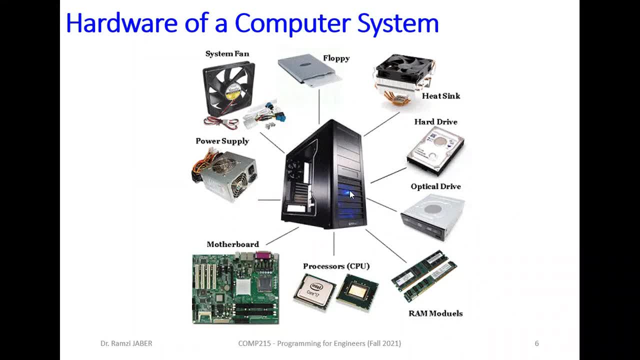 and so on in the case in the case we have inside it of course fan one fan or two fan and of course to generate to operate all these components we need power supply so power supply will convert the ac power 220 volt the ac 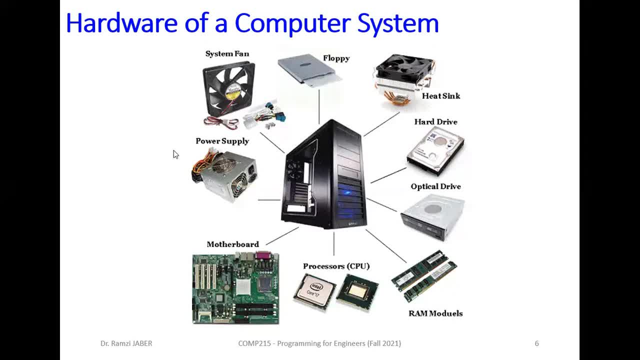 power from your home to 120 volts converted to dc power from ac to dc from ac power 220 volts to dc power dc volt like for the motherboard 5 volts for the ram 3.3 volts from the dvd rom or hard disk or fans will be 12 volt so the power supply has many outputs dc zero volt of course 3.3 volts for rams and some vga some vga needs are also 3.3 volts 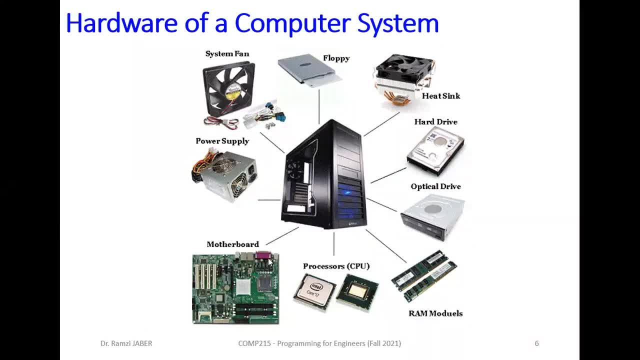 also we have 5 volts for the motherboard and 12 volt for mechanical parts for mechanical parts 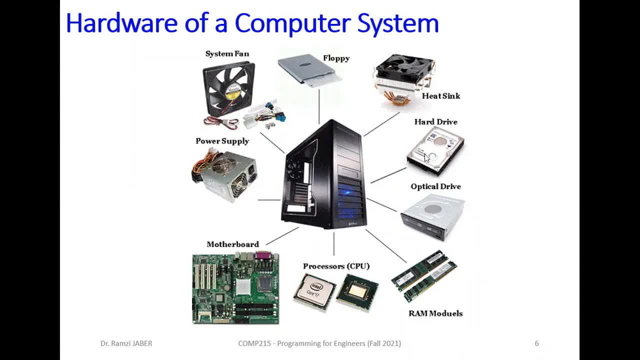 means for fans all the hard disk all the hard disk and optical drive okay now do you have any question for this do you have any question for this slide 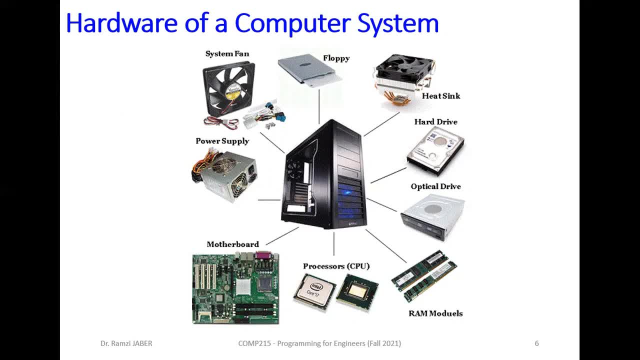 good no so now we'll go to the software as you know so now we'll go to the software as you know 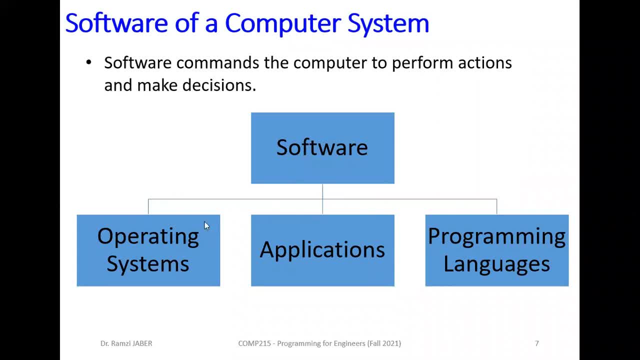 so now we'll go to the software as you know the software the software the software also decomposed for three also decomposed for three also decomposed for three parts operating system parts operating system parts operating system like windows ios and so on like windows ios and so on like windows ios and so on applications applications applications software applications like word excel software applications like word excel software applications like word excel powerpoint and so on and so on powerpoint and so on and so on powerpoint and so on and so on photoshop and so on games and so on 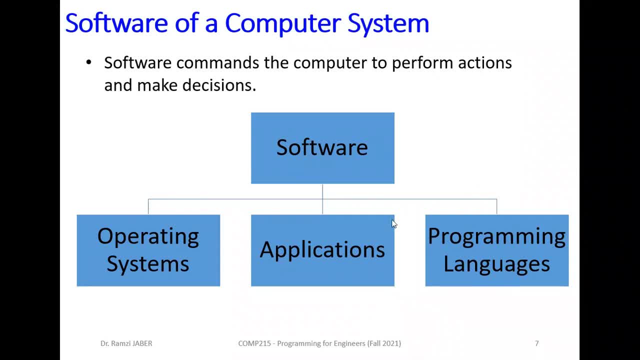 photoshop and so on games and so on photoshop and so on games and so on also the programming language languages 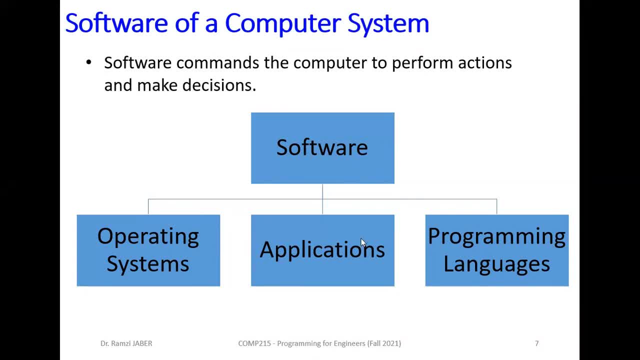 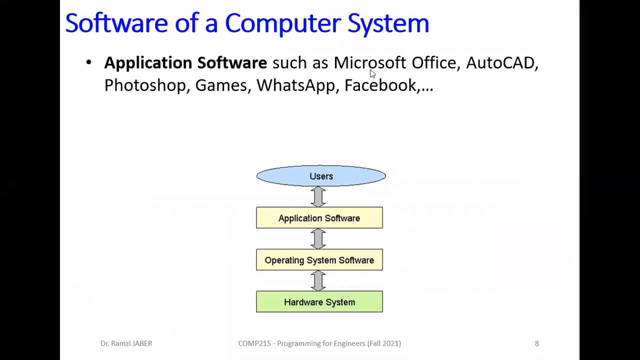 the application software which is which is which is any application you have any application you have any application you have like microsoft office autocad photoshop like microsoft office autocad photoshop like microsoft office autocad photoshop games whatsapp facebook and and and and games whatsapp facebook and and and and games whatsapp facebook and and and and and so this is called application software and so this is called application software and so this is called application software so the user so the user so the user will use this application software one of will use this application software one of will use this application software one of them any application software them any application software 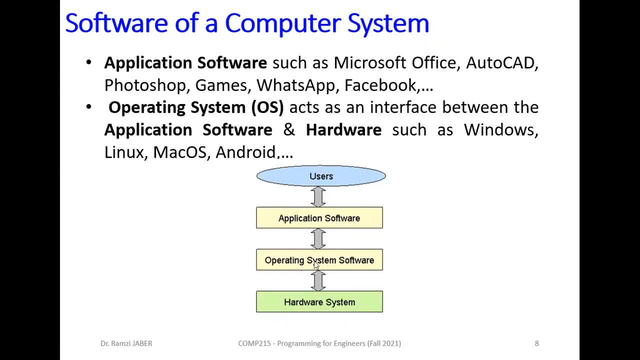 them any application software the operator operating system software the operator operating system software the operator operating system software the operating system like the operating system like the operating system like windows windows windows linux mac os ios android and so on linux mac os ios android and so on linux mac os ios android and so on acts this operating system acts as an acts this operating system acts as an acts this operating system acts as an interference or interface between the interference or interface between the interference or interface between the application software and the hardware application software and the hardware 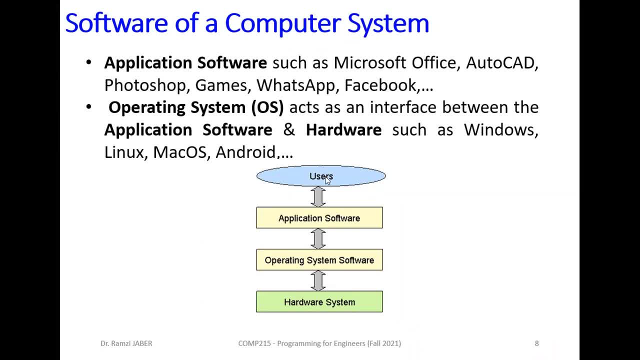 application software and the hardware system system system okay so okay so okay so the user will use an application 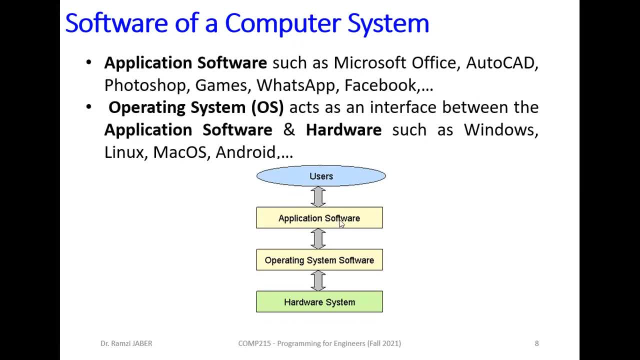 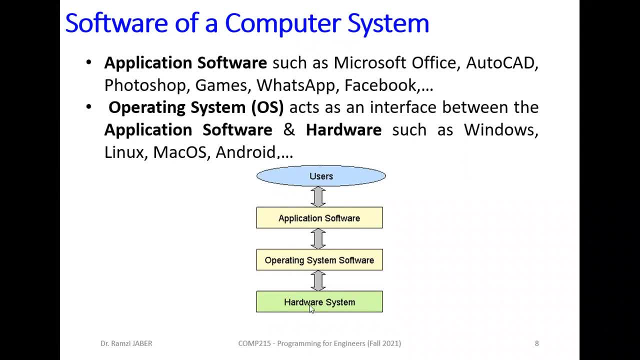 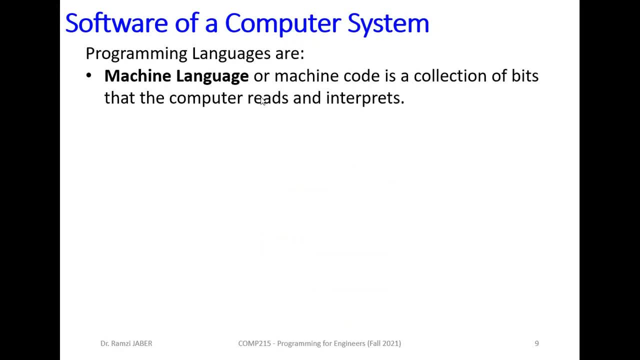 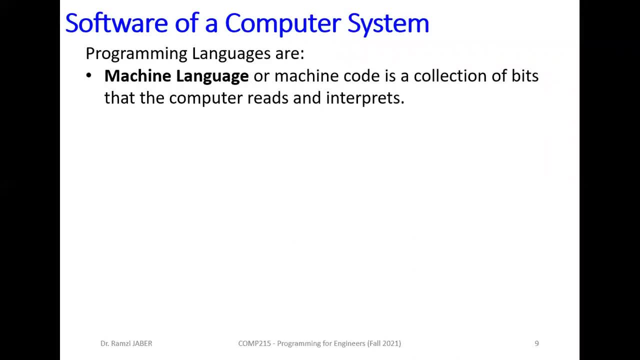 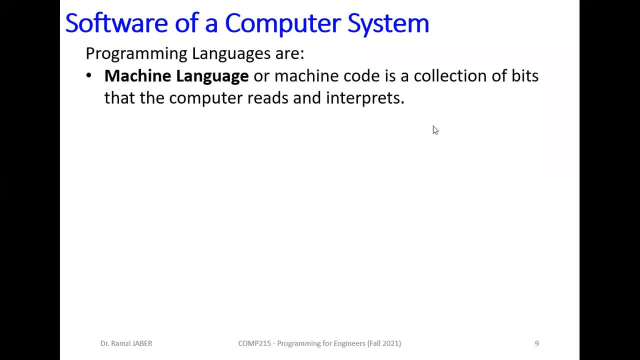 so i write it or i put it zero zero so i write it or i put it zero zero one one zero one zero one whatever so it's one one zero one zero one zero one whatever so it's one one zero one zero one zero one whatever so it's series of series of 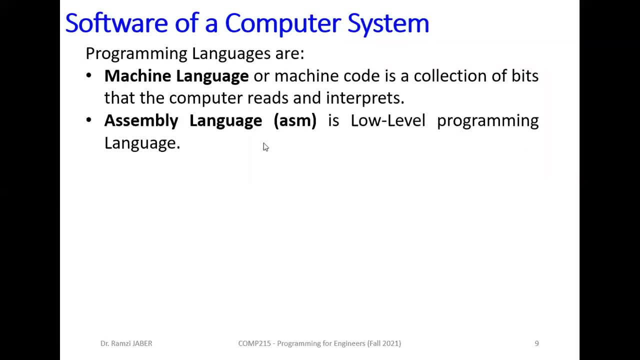 series of switches this is machine language switches this is machine language switches this is machine language later later 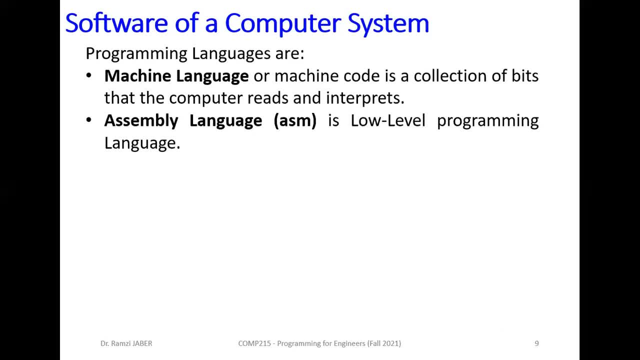 later later they invent later they invent later they invent a low level programming language low a low level programming language low a low level programming language low level programming language it's assembly level programming language it's assembly 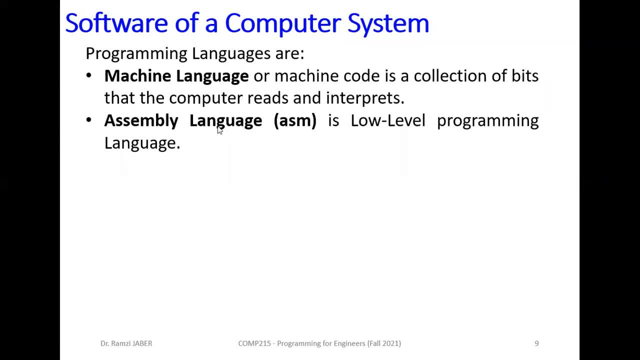 level programming language it's assembly language language language acm acm acm asm assembly language asm assembly language asm assembly language also also also it's hard it's not easy like it's hard it's not easy like it's hard it's not easy like today python okay it's hard language today python okay it's hard language today python okay it's hard language you can you can you can use some 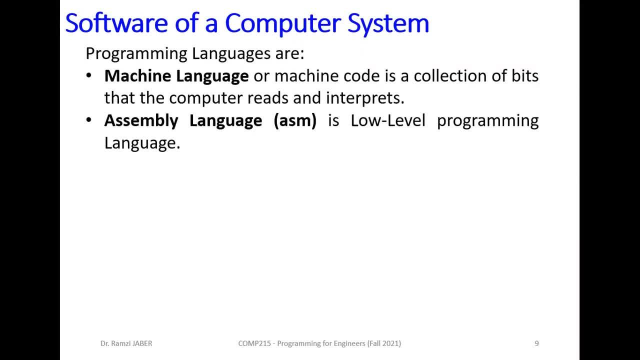 use some use some english commands but still hard english commands but still hard english commands but still hard inside any language we have 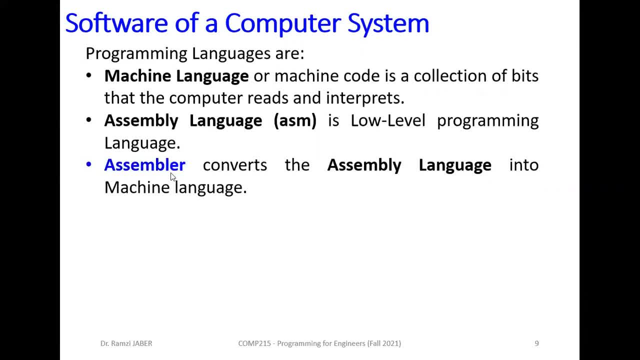 something like assembler something like assembler something like assembler assemblers assemblers assemblers convert the assembly language convert the assembly language convert the assembly language into machine language into machine language 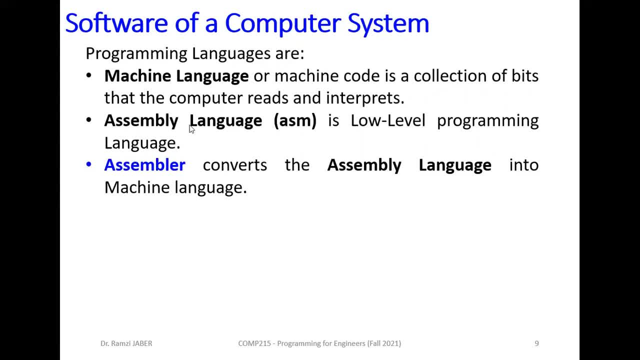 into machine language so to convert this syntax so to convert this syntax so to convert this syntax some english word inside assembly 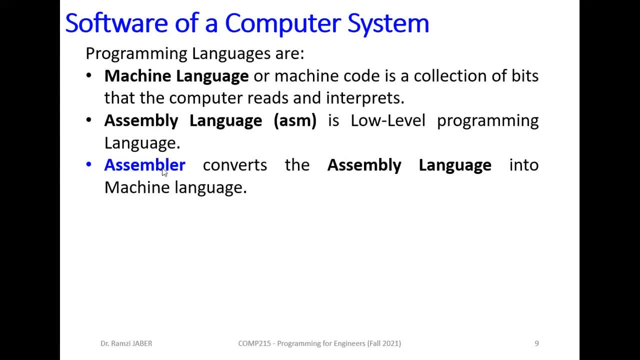 some english word inside assembly some english word inside assembly language to the machine language language to the machine language language to the machine language we need assembler we need assembler 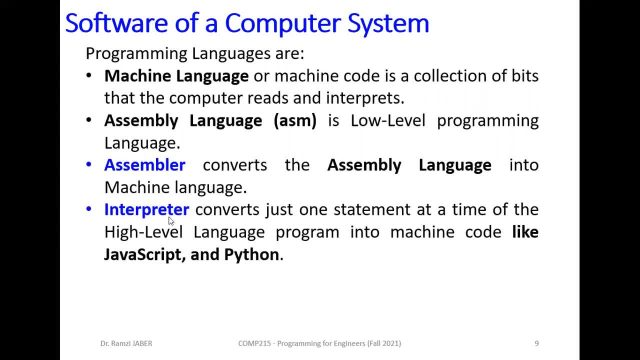 we need assembler we have also something called interpreter we have also something called interpreter we have also something called interpreter interpreter interpreter interpreter also it's also it's also it's like like like engine or libraries converts engine or libraries converts 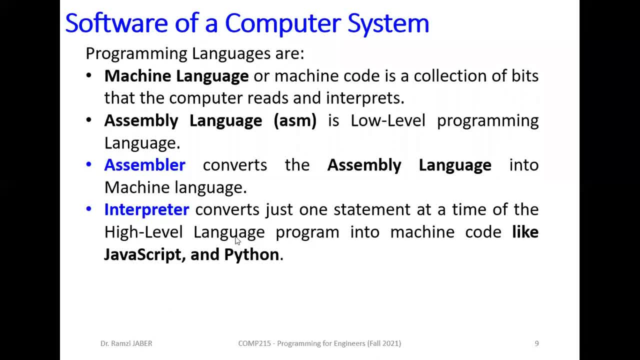 engine or libraries converts just one statement at the time of the just one statement at the time of the just one statement at the time of the high level language high level language high level language program into machine code or machine program into machine code or machine program into machine code or machine language language language like javascript and python c's okay so like javascript and python c's okay so like javascript and python c's okay so interpreter it's similar to interpreter it's similar to interpreter it's similar to javascript and python so python it's not javascript and python so python it's not javascript and python so python it's not compiler 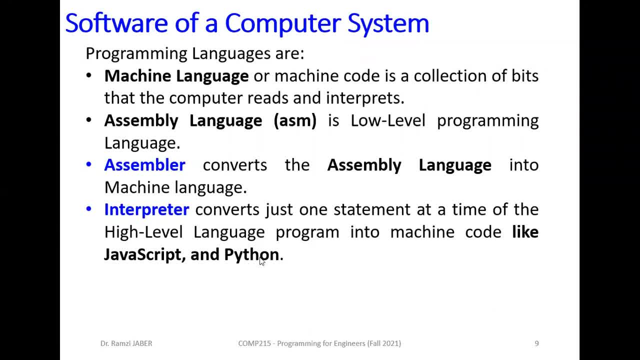 compiler compiler c is compiler python is not compiler c is compiler python is not compiler c is compiler python is not compiler it's interpreter programming language 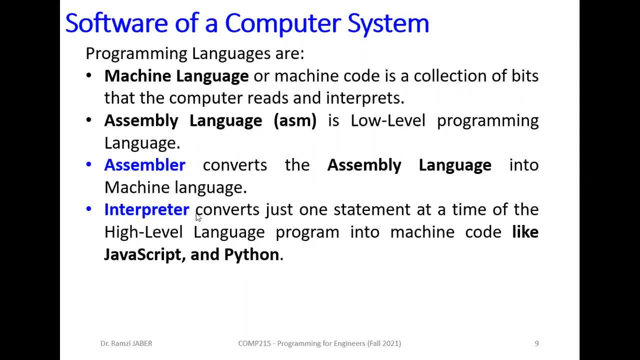 it's interpreter programming language it's interpreter programming language so python it's interpreter so python it's interpreter so python it's interpreter programming language programming language 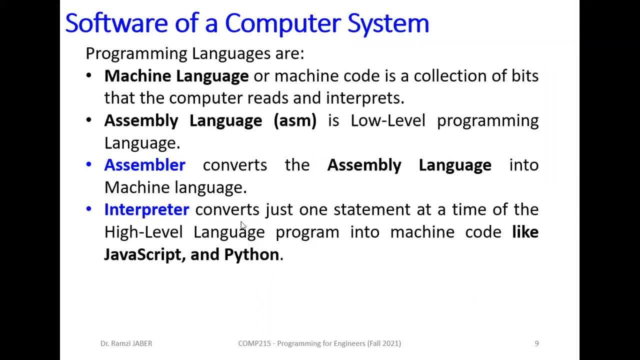 programming language the interpreter inside python the interpreter inside python the interpreter inside python will will will convert one syntax by one syntax one convert one syntax by one syntax one 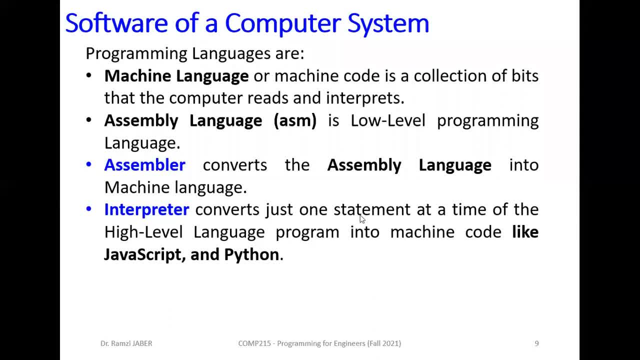 convert one syntax by one syntax one line by one line line by one line line by one line okay statement by statement if an error okay statement by statement if an error okay statement by statement if an error occur occur occur so the error will be halt or paused for so the error will be halt or paused for so the error will be halt or paused for this line to be corrected this line to be corrected this line to be corrected okay so it's slower okay so it's slower okay so it's slower for error for checking error it's slower for error for checking error it's slower for error for checking error it's slower than compiler than compiler than compiler and we have compiler scans the entire and we have compiler scans the entire and we have compiler scans the entire programs programs programs and converts the whole high level and converts the whole high level and converts the whole high level language into machine code like language into machine code like language into machine code like c c plus plus and java so i will repeat c c plus plus and java so i will repeat c c plus plus and java so i will repeat again what is again what is again what is the difference between compiler and the difference between compiler and 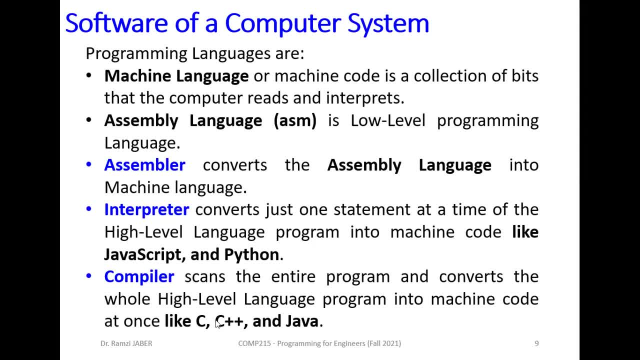 the difference between compiler and interpreter okay interpreter okay interpreter okay like c and c plus plus and java like c and c plus plus and java like c and c plus plus and java the compiler for checking for error when the compiler for checking for error when the compiler for checking for error when you convert your code your english code you convert your code your english code you convert your code your english code to the machine code okay to the machine code okay to the machine code okay in the compiler they scan all the code in the compiler they scan all the code in the compiler they scan all the code your codes and state your errors your codes and state your errors your codes and state your errors the errors inside your code so the errors inside your code so the errors inside your code so first step write your code second step first step write your code second step 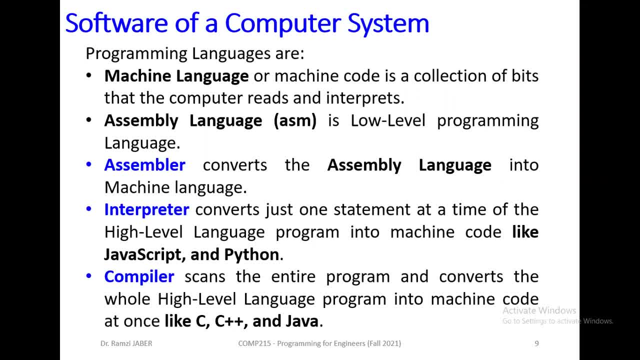 first step write your code second step checking your code for errors in checking your code for errors in checking your code for errors in compiler when in checking errors compiler when in checking errors compiler when in checking errors your code for errors your code for errors your code for errors will list you lot of errors in will list you lot of errors in will list you lot of errors in in this line that line and that line so in this line that line and that line so in this line that line and that line so you can correct them update your code you can correct them update your code 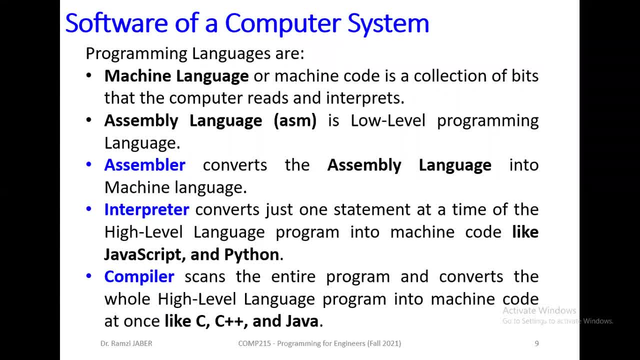 you can correct them update your code save it and run again whereas it's 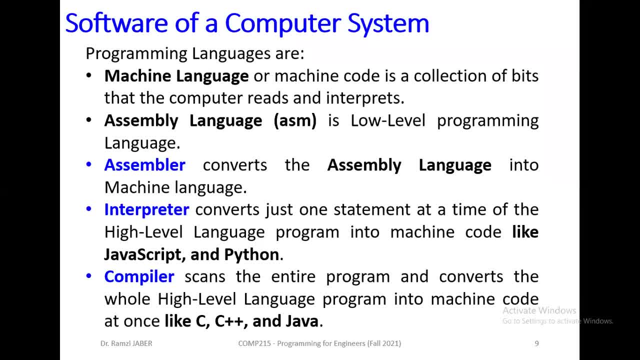 save it and run again whereas it's save it and run again whereas it's faster than interpreter faster than interpreter faster than interpreter for checking for errors compiler is for checking for errors compiler is for checking for errors compiler is faster faster faster okay so and and inside interpreter like 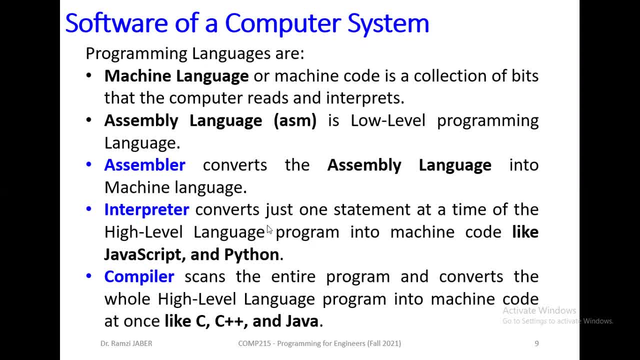 okay so and and inside interpreter like okay so and and inside interpreter like python python python the when you run checking for errors in the when you run checking for errors in the when you run checking for errors in python 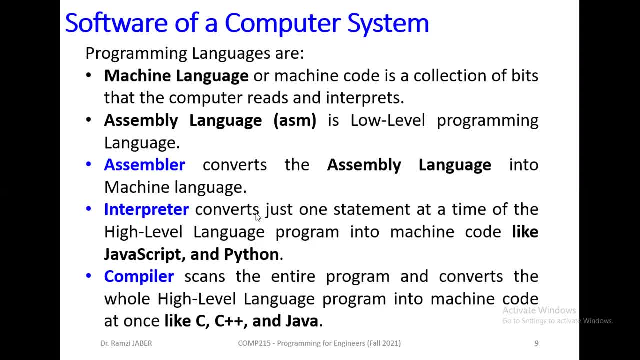 python python the interpreter will checking line by the interpreter will checking line by the interpreter will checking line by line statement by statement if another line statement by statement if another line statement by statement if another occurred will stop occurred will stop occurred will stop and state for you that is error you need and state for you that is error you need and state for you that is error you need to to to update it correct it then run again run update it correct it then run again run update it correct it then run again run again run again again run again run again again run again run again if you have lots of errors if you have lots of errors 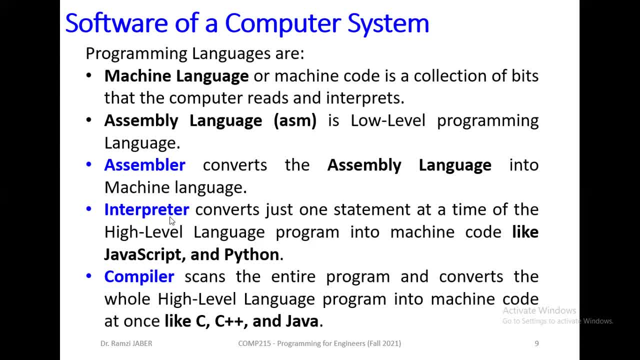 if you have lots of errors of course compilers faster than of course compilers faster than of course compilers faster than interpretable interpretable interpretable but but 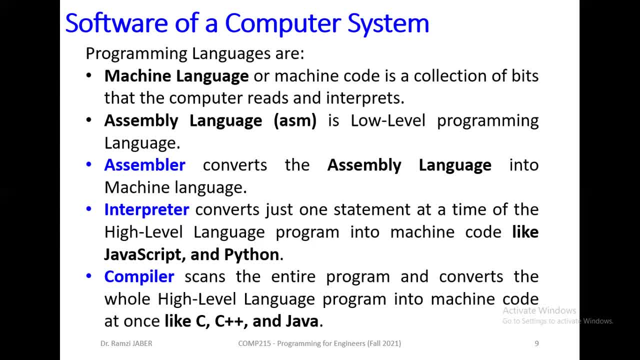 but but for running programs but for running programs but for running programs if you if you write code in python or if you if you write code in python or 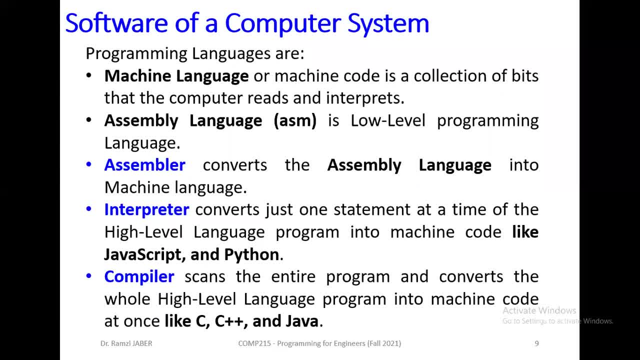 if you if you write code in python or nc without errors without errors nc without errors without errors nc without errors without errors the interpreter is faster than compiler the interpreter is faster than compiler the interpreter is faster than compiler for 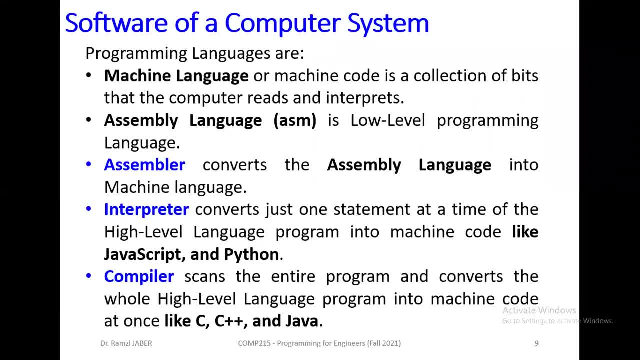 for for running for execution file to convert it running for execution file to convert it running for execution file to convert it to the machine code and execution file to the machine code and execution file 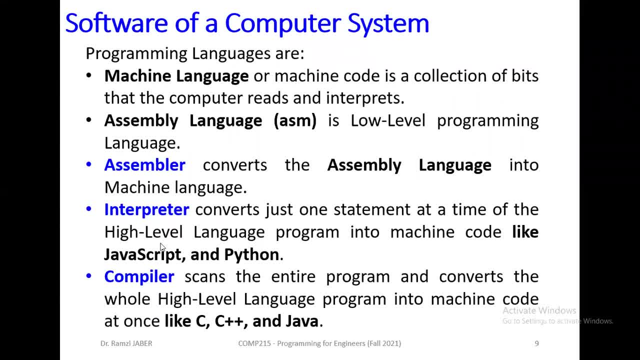 to the machine code and execution file to be run your application so python or to be run your application so python or to be run your application so python or interpreter not only python the interpreter not only python the 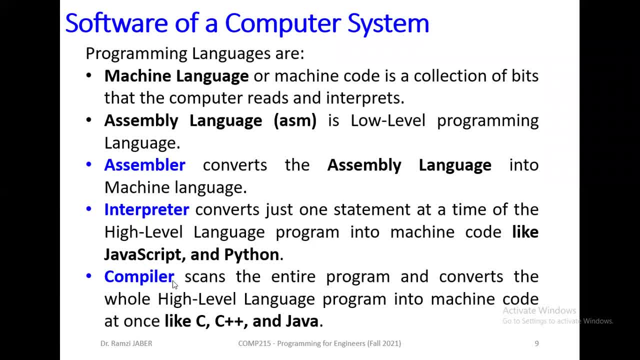 interpreter not only python the interpreter is faster than compiler interpreter is faster than compiler interpreter is faster than compiler but it's slower but it's slower 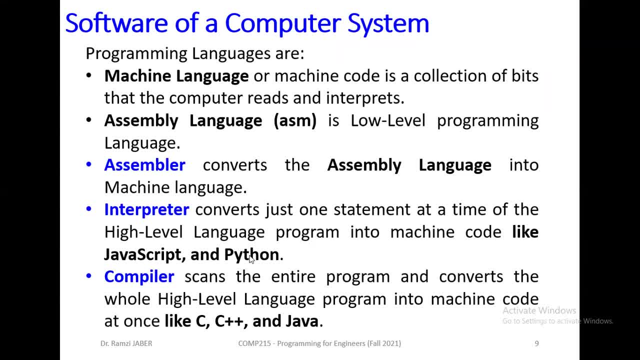 but it's slower when checking for errors okay when checking for errors okay when checking for errors okay you got the ideas any question here 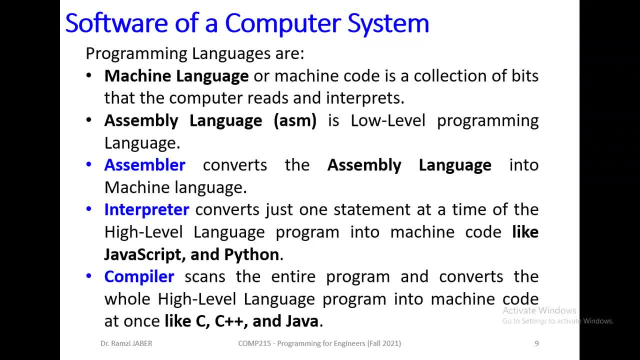 good doctor good doctor good doctor 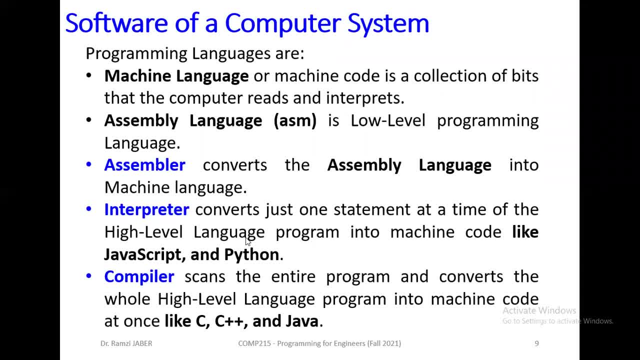 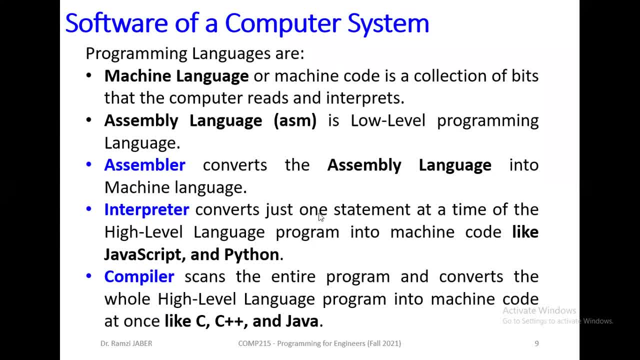 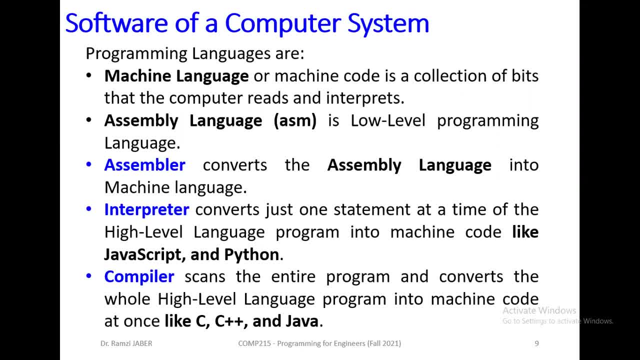 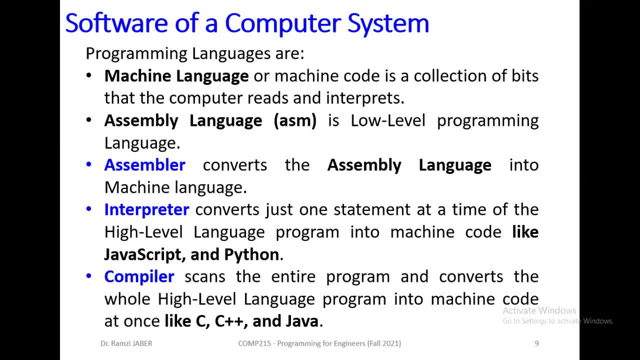 checking for errors the compiler is faster than the interpreter meanwhile interpreter meanwhile interpreter meanwhile meanwhile after that meanwhile after that meanwhile after that if you don't have a mistake no no errors if you don't have a mistake no no errors if you don't have a mistake no errors in your codes in your codes in your codes interpreter is faster than compiler interpreter is faster than compiler interpreter is faster than compiler okay good good 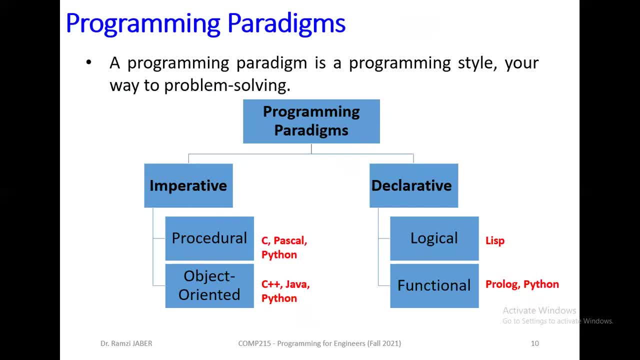 good now we have different paradigm now we have different paradigm now we have different paradigm style paradigm means style style paradigm means style style paradigm means style who is time who is time 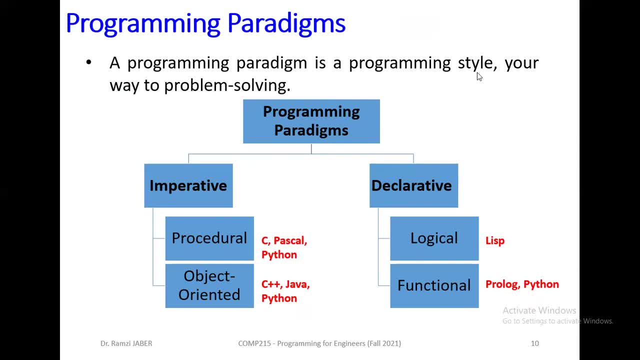 who is time a programming paradigm is a programming a programming paradigm is a programming a programming paradigm is a programming style style style it's loop it's loop it's loop how to write how to write how to write your way to problem solving how to think your way to problem solving how to think your way to problem solving how to think what is your algorithm 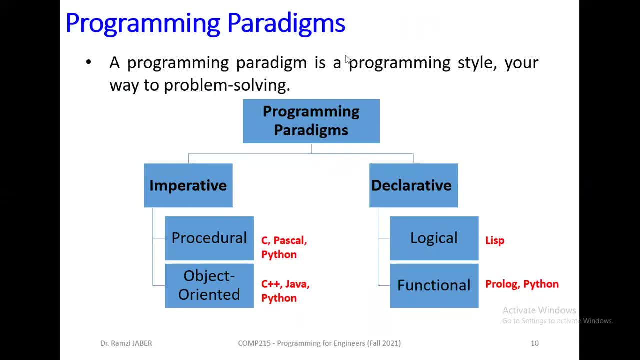 what is your algorithm what is your algorithm okay this is called the style okay this is called the style okay this is called the style so paradigm we have so paradigm we have so paradigm we have different paradigm in any programming different paradigm in any programming different paradigm in any programming language language language okay okay okay we have programming paradigm we have we have programming paradigm we have we have programming paradigm we have imperative and declarative imperative and declarative 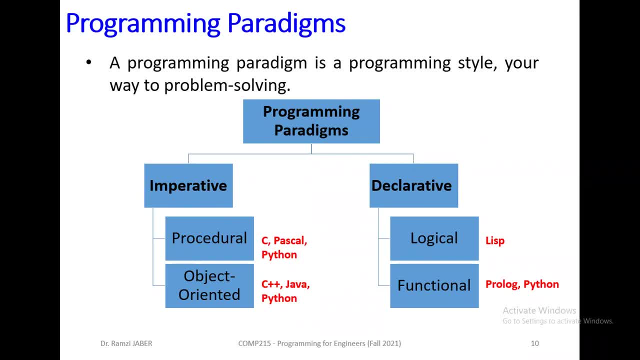 imperative and declarative imperative means you have a fixed imperative means you have a fixed imperative means you have a fixed algorithm fixed steps to do step one i algorithm fixed steps to do step one i algorithm fixed steps to do step one i want to do this step two i want to do want to do this step two i want to do want to do this step two i want to do that step three step four so it's that step three step four so it's that step three step four so it's in details in details in details imperative means you write your code in imperative means you write your code in imperative means you write your code in a procedural way a procedural way a procedural way procedural way step one step two sub three 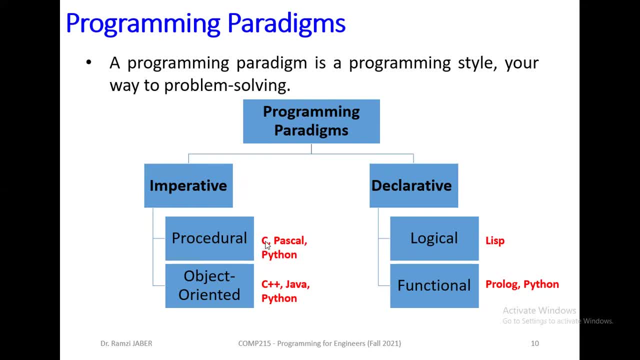 procedural way step one step two sub three procedural way step one step two sub three step four sub five okay like you did step four sub five okay like you did step four sub five okay like you did and see and see 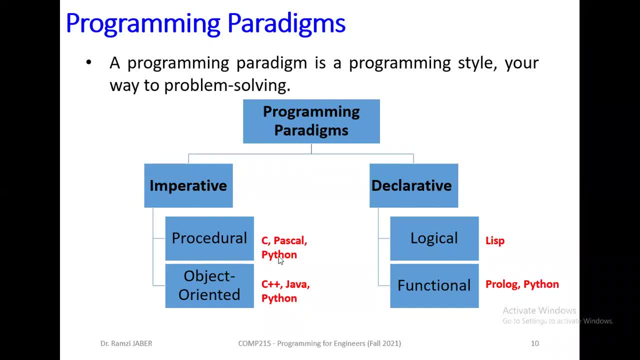 and see also python has this function also python has this function also python has this function this paradigm this paradigm 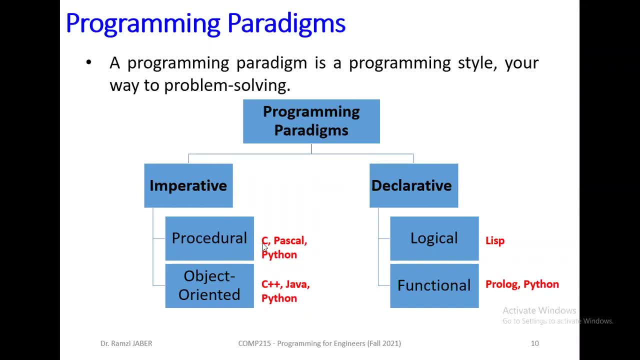 this paradigm okay so procedures language is like c okay so procedures language is like c okay so procedures language is like c pascal python pascal python pascal python also we have object oriented also we have object oriented 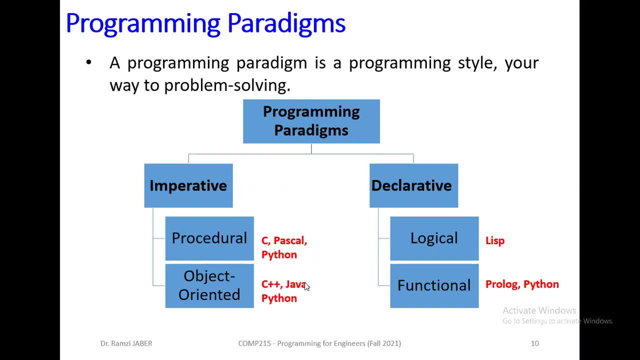 also we have object oriented if you get if you get if you get op course op course op course you will use java you will use java you will use java or c plus plus or c plus plus or c plus plus so c plus plus java is object oriented so c plus plus java is object oriented so c plus plus java is object oriented also it's imperative language also it's imperative language also it's imperative language also as you can see also as you can see also as you can see we have python 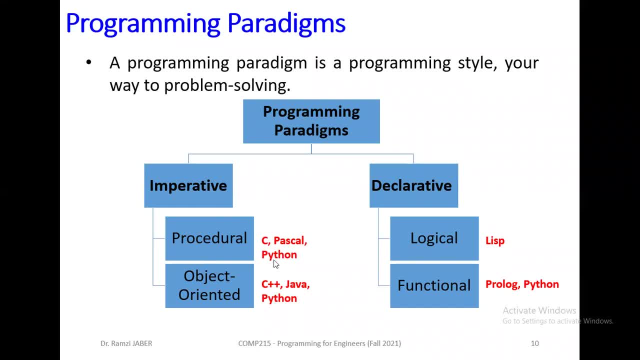 we have python we have python so python so python so python is procedure is procedure is procedure and and and object oriented object oriented object oriented also functionally okay so the first also functionally okay so the first also functionally okay so the first part part part for step one step two sub three in for step one step two sub three in for step one step two sub three in details structures and details writing a details structures and details writing a details structures and details writing a syntax syntax syntax called imperatives called imperatives called imperatives and we have declarative 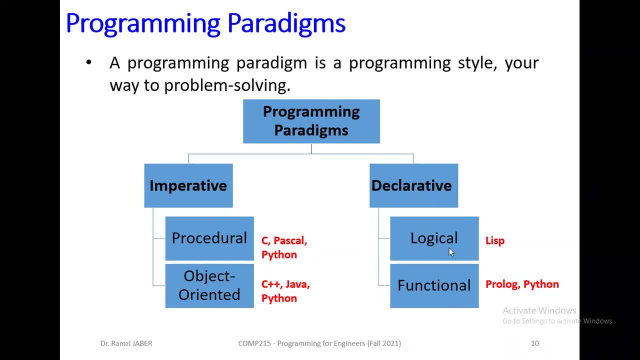 and we have declarative and we have declarative paradigm declarative paradigm like paradigm declarative paradigm like paradigm declarative paradigm like logical functions logical functions 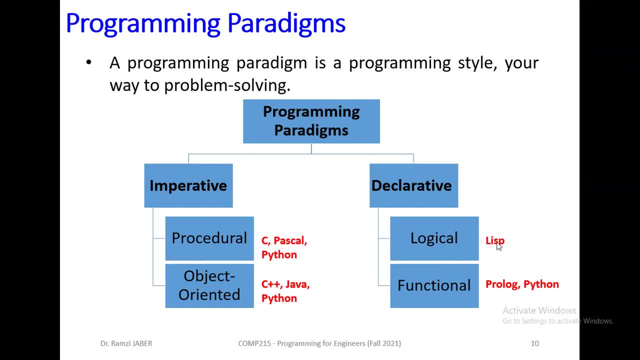 logical functions or logical thinking or logical thinking or logical thinking like language called list 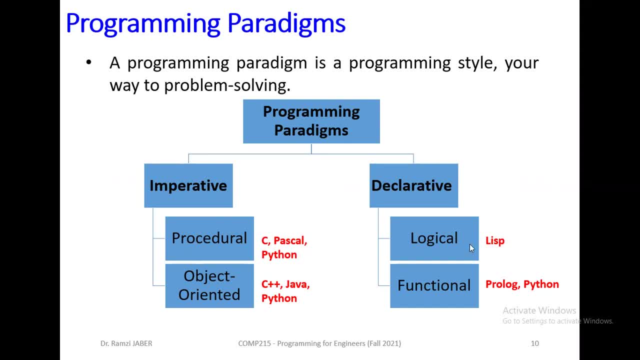 like language called list like language called list we have a language called list we have a language called list we have a language called list used for logical used for logical used for logical thinking okay 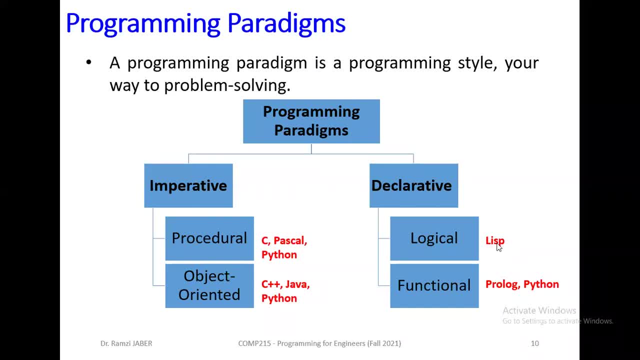 in in 2014 in in 2014 in in 2014 we stopped in beirut arab university we stopped in beirut arab university we stopped in beirut arab university teach list teach list teach list okay okay okay in the old days and all year in the old 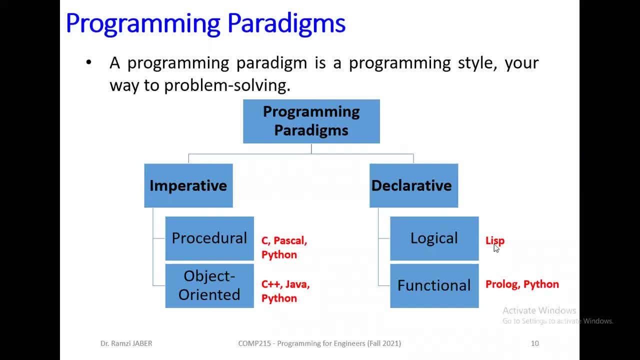 in the old days and all year in the old in the old days and all year in the old years we teach years we teach years we teach list inside beirut arab university okay list inside beirut arab university okay 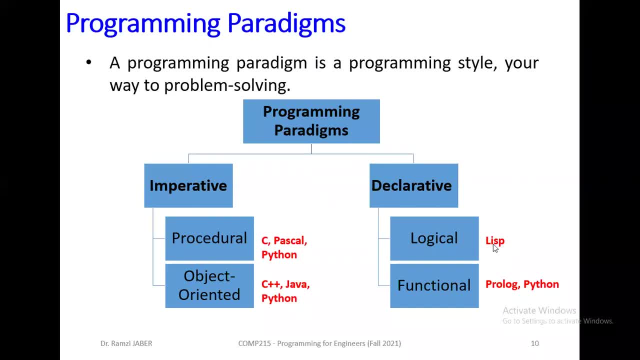 list inside beirut arab university okay but 2014 and but 2014 and but 2014 and till now we stopped list okay till now we stopped list okay till now we stopped list okay so it's logical so it's logical so it's logical thinking thinking thinking uh uh 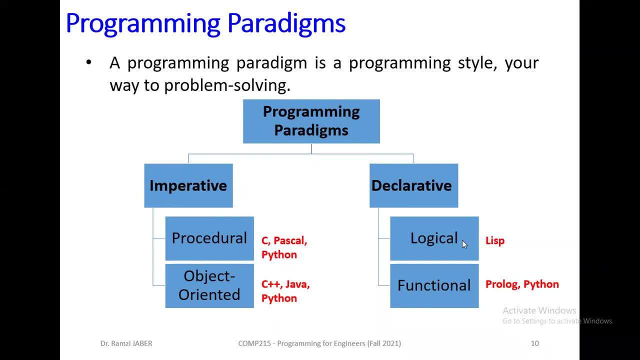 uh language it's like english language it's language it's like english language it's language it's like english language it's like pseudocode similar to pseudocode like pseudocode similar to pseudocode like pseudocode similar to pseudocode write in english write in english write in english statements then converted to the statements then converted to the statements then converted to the machine code machine code machine code also we have functional also we have functional also we have functional language functional language like language functional language like language functional language like prologue 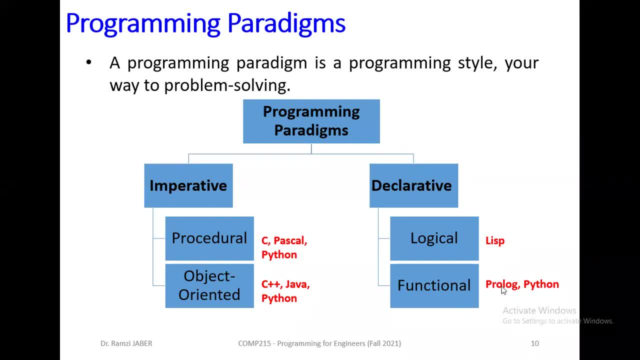 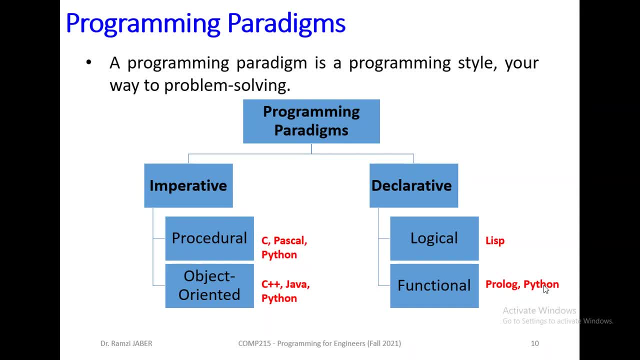 okay now the functional will be the functional will be the functional will be today is python so as you can see today is python so as you can see today is python so as you can see python at the same time python at the same time python at the same time has different style has different style has different style you can use it as functional language you can use it as functional language you can use it as functional language and you can use it as procedural and you can use it as procedural and you can use it as procedural language or as oop language so this is language or as oop language so this is language or as oop language so this is why python is dominate 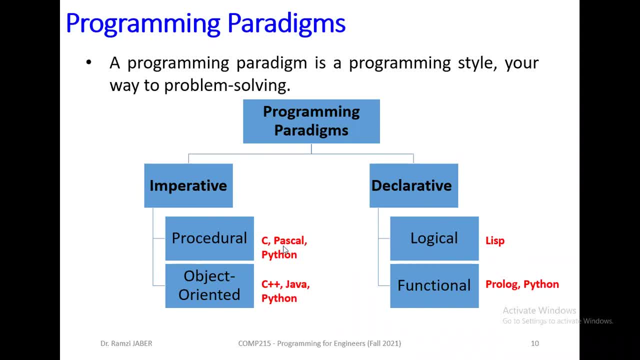 why python is dominate why python is dominate that's why python is dominate on all that's why python is dominate on all that's why python is dominate on all other programming language because you other programming language because you other programming language because you can use it as functional you can use it can use it as functional you can use it can use it as functional you can use it as op also you can use it as a procedural as op also you can use it as a procedural as op also you can use it as a procedural so that's why python is very dominate so that's why python is very dominate so that's why python is very dominate right now in these years right now in these years right now in these years okay okay so we will learn in this course 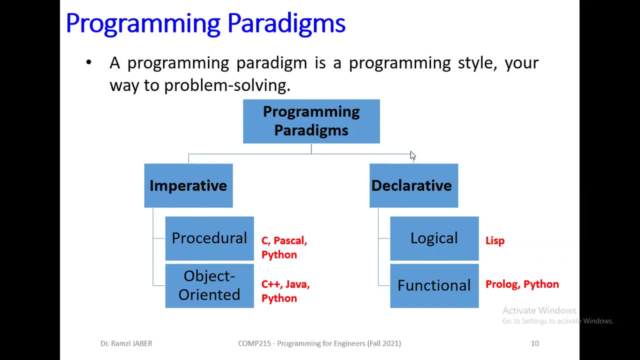 okay okay so we will learn in this course python python python any question for this slide 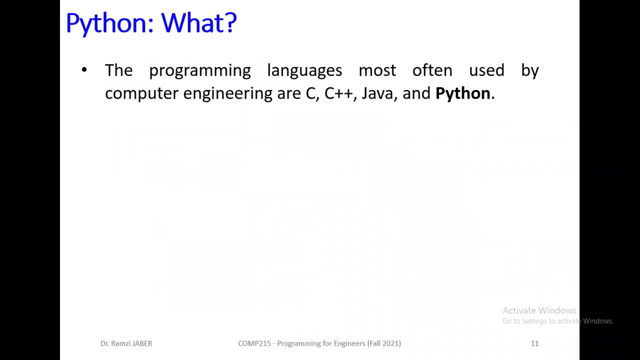 good now now now now becomes python becomes python becomes python 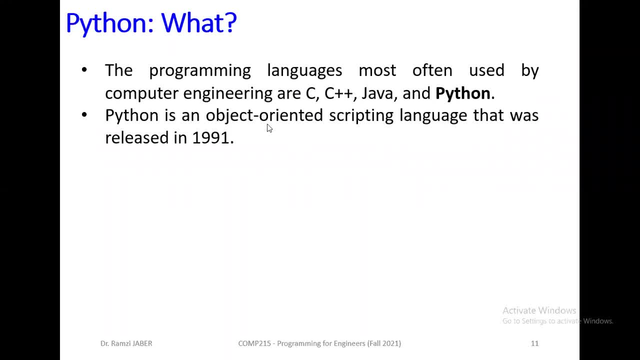 okay python is an op object-oriented scripting language that was released in 91 but it's not famous indeed in that year starting 81 and 91 sorry 1991 but it's not very famous at this year at that year it was developed by judo of the national research institute for mathematical and computer science in amsterdam so it's from amsterdam the first issues or version for python so python has rapidly become one of the world's most popular programming languages 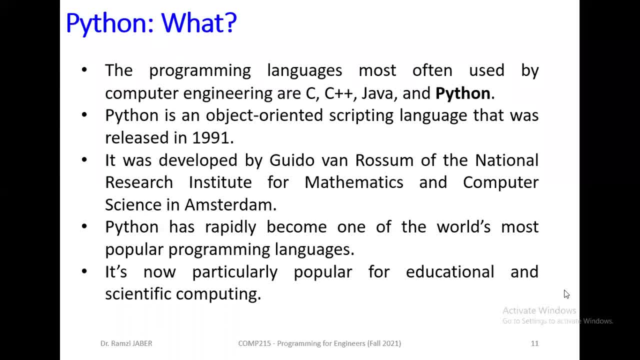 it's now particularly popular for educational and scientific computing they use python in educational programming language and for scientific 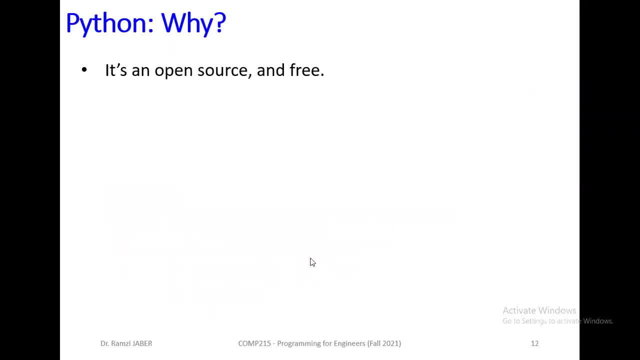 programming languages it's a free programming language it's not like others not like other programming languages like microsoft visual visual c plus plus visual basics and so on asp and so on and so on so it's a free programming language 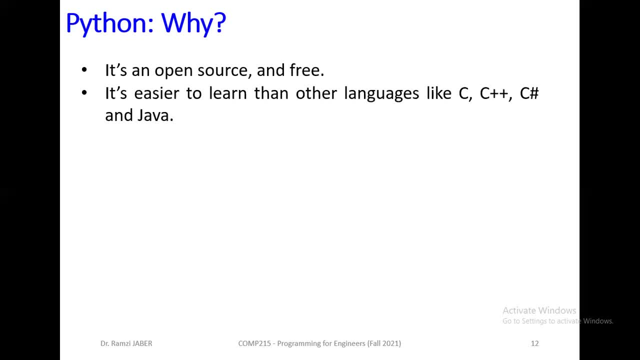 it's easier to learn than other languages like c c plus plus c sharp and java it's simpler easier simpler we have built-in functions we can use it directly so it's easier 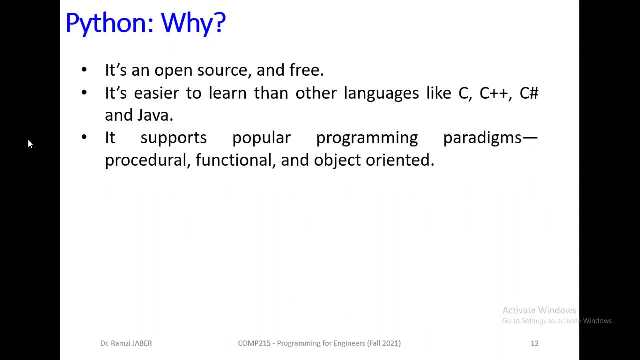 it supports popular programming paradigm procedure functional and op object oriented as we said before it enhances developer productivity with extensive standard libraries we have in python extensive libraries we have many many many libraries and thousands of third-party open libraries 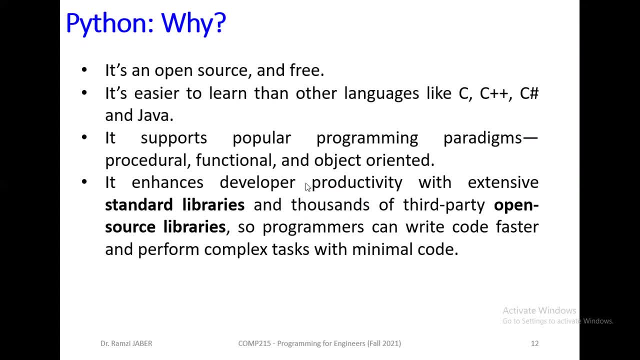 thousands okay so we have many libraries so programmers can write code faster and perform complex tasks with minimal code just use any build-in function or libraries you can use it directly no need to to reinvent the wheel just use existing libraries or functions 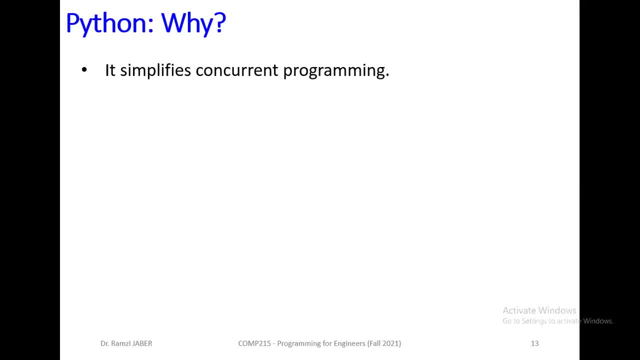 why we want to use python because it simplifies concurrent programming 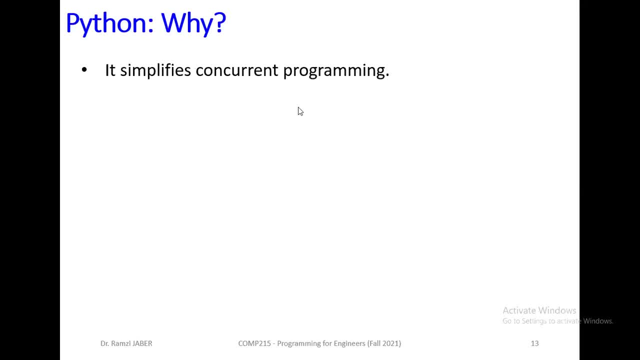 concurrent programming means parallel programming you can you can run running or execute your programs in parallel way there is some libraries some code inside python that can your code can be running in parallel for parallel cpu in c it's very hard okay in c plus 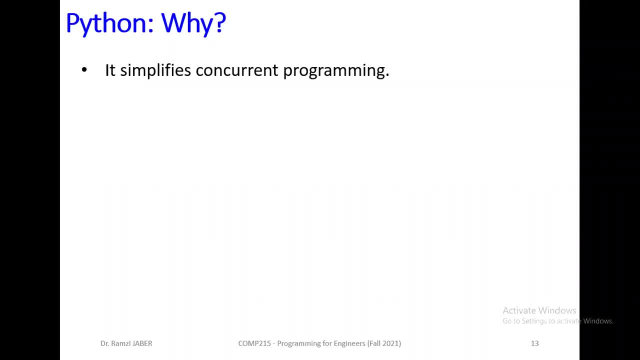 plus we have okay in java we have parallel so because we can use it as parallel programming language this is advantage 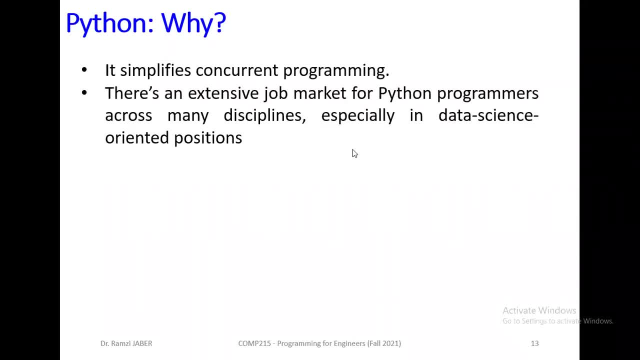 also we can use extensive job market because right now if you search for a job for programming job or software engineer jobs inside u.s europe or all the world 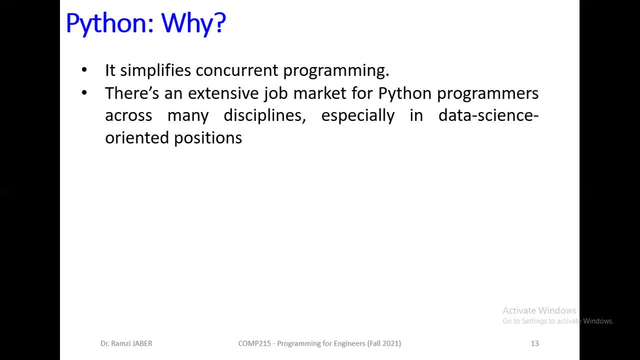 every job description has include python you know python we will hire you okay so python is right now booming in all companies 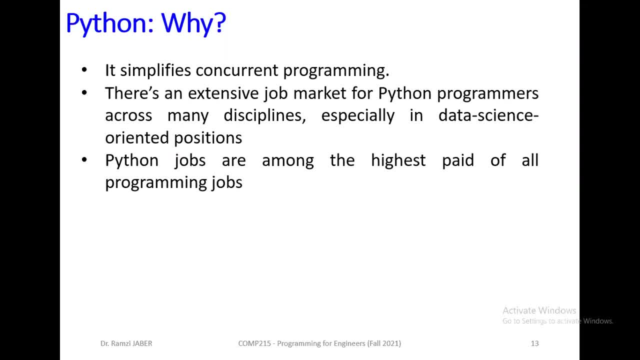 also also the the python jobs are among the highest paid of all programming jobs also when you search by google you can see the top salaries in software engineer is python where is python we can use python where 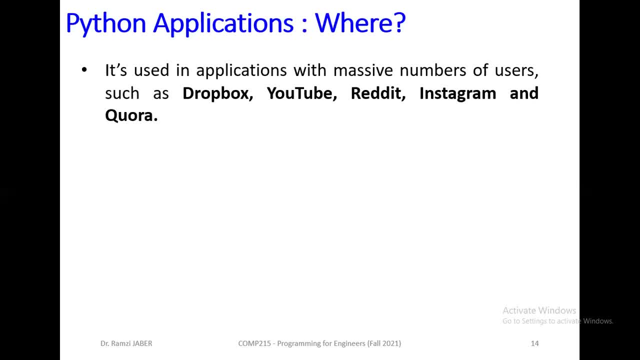 of course you can use python in applications with the massive number of users which other language cannot like c c plus plus cannot be programmed 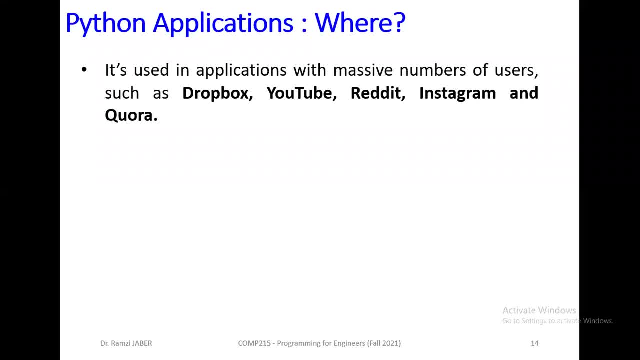 for massive number of users on the global internet such as dropbox youtube reddit instagram and quora 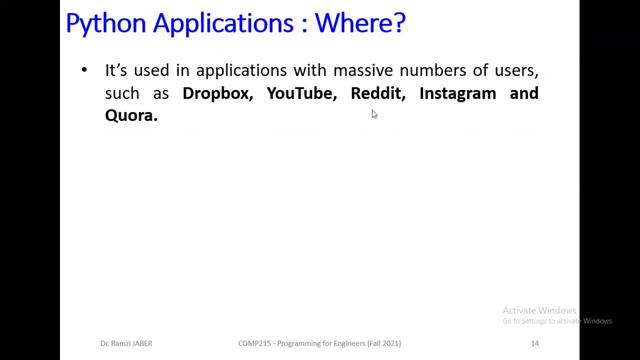 and also others others so these platforms or these websites as you can see using python youtube 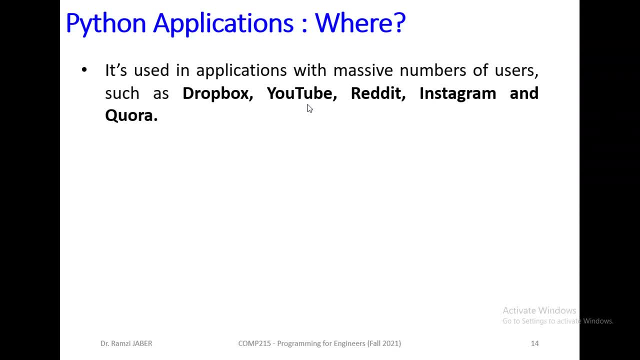 itself the code of youtube is python okay of course python can be used as web development development like jaguar and flask they use python also youtube they use python in the game game 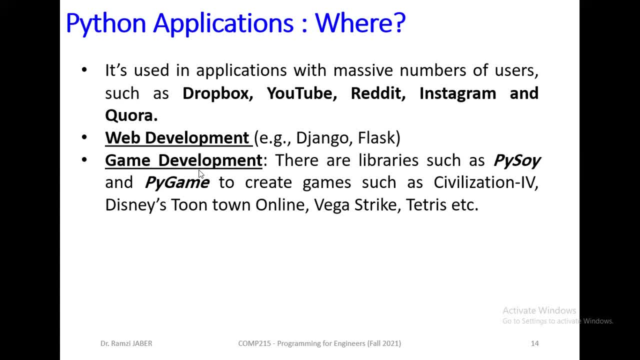 development so you can use python in the game there are libraries such as pisol or pygame to create games such these games disney town vega tetris etc etc etc so python you can create a game 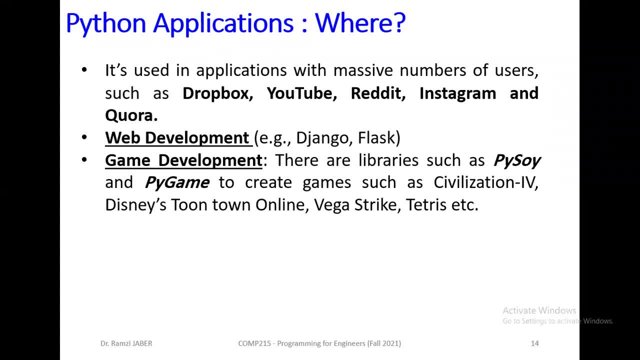 and we will make a game at the end of the course at the end of the course we want to create a small application and small games of course for the highest peak or topics in the world is machine 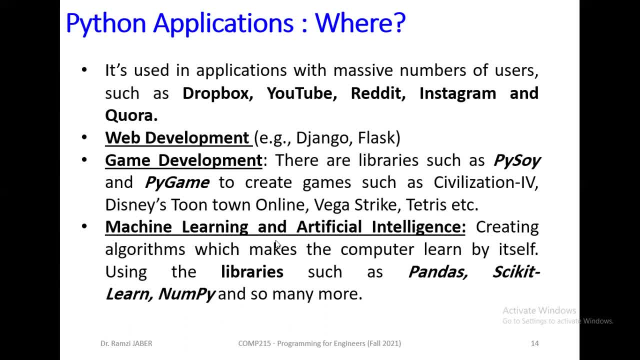 learning and artificial intelligence so these topics becomes nowadays booming so they use also creating algorithm which makes the computer learn by itself using the libraries such as pandas 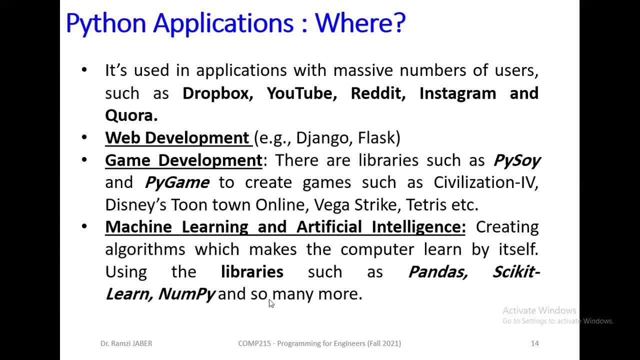 and numpy and so many others okay also we use python in artificial intelligence and machine learning 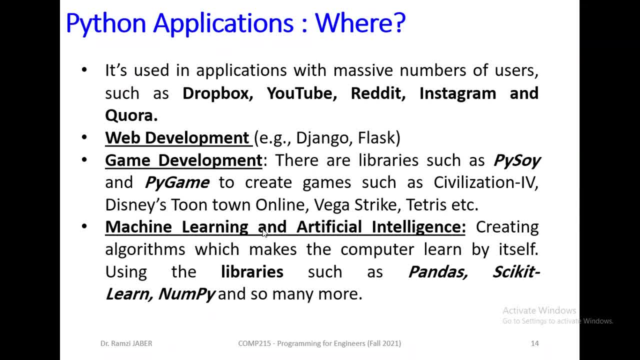 which are hot topics in these days using python 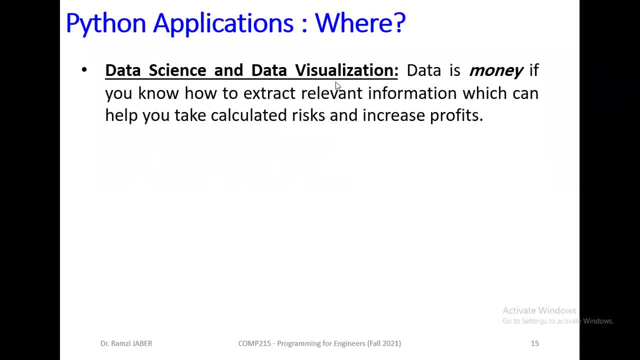 also in data science and data visualization like data is money if you know how to extract prevalent information which can help you take calculated risk and increase the 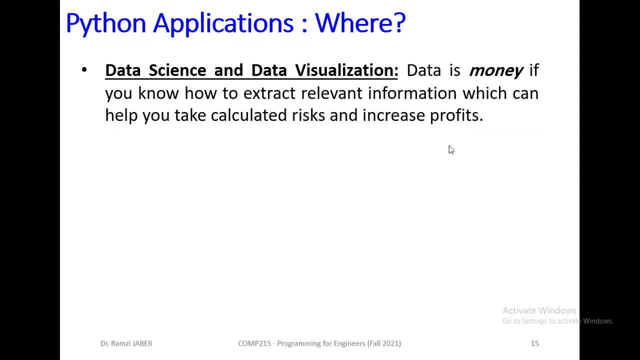 asm Preferred benefit so insert in statistical website 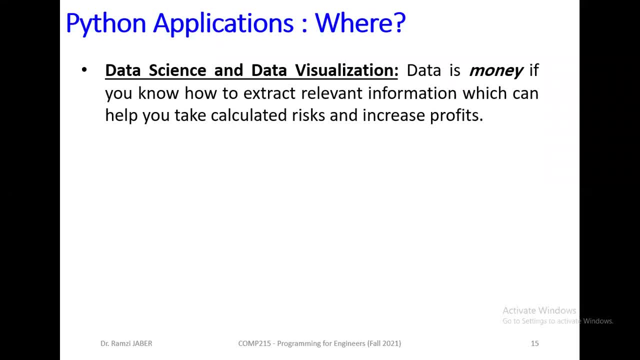 analysis reports Python makes reports and upward statistics works as a mathematical application 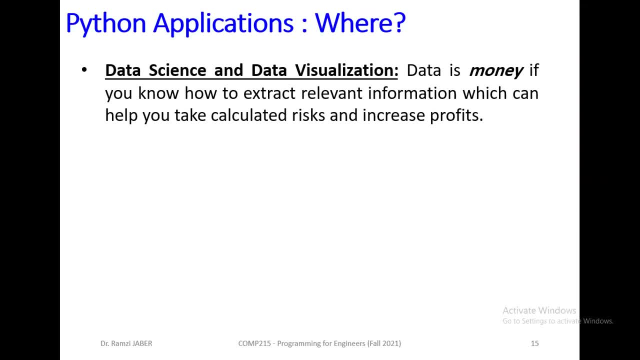 faster than accessibility programs how to make statist relevant and donc Eating to cure having foods faster than mamy fast than Undert › Buramish fast than other programs fast thanying fast polsk 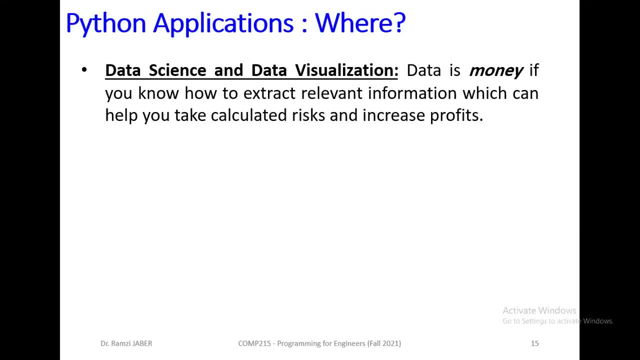 fast from websites fast from votre to save money in the program fast from internet this is fast from internet very important 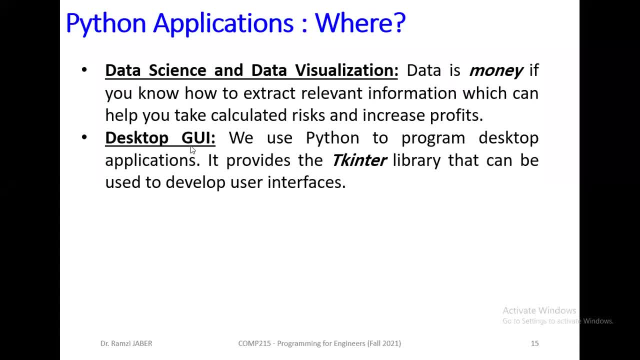 also we have gi graphical user interface we use python to program desktop application 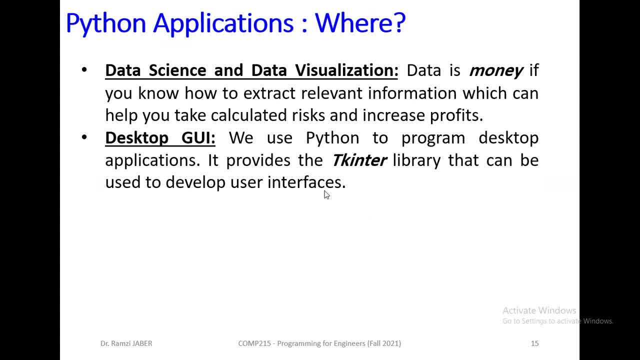 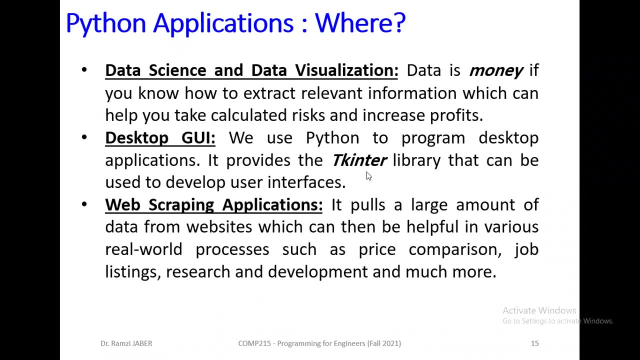 like tick enter library that can be used to develop user interface we will use this library after meter okay after meter will you will begin gi graphical user interface tick enter we will make some application and some game using tick enter also in the web applications 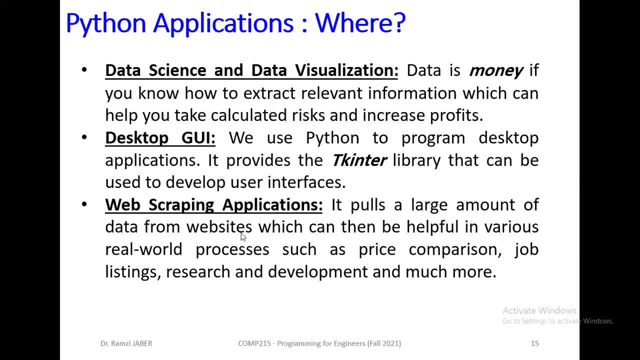 so it puts a large amount of data from websites which can then be helpful in various real world processes such as the price comparison as we said before data science and data visualization jobs listening research and development and much more so we can use python in everywhere everywhere 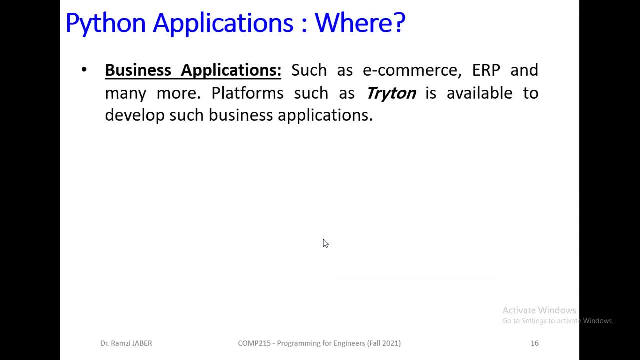 everything also in business applications just as e-commerce erp and many more platforms such as triton is available to develop such business applications like in alibaba 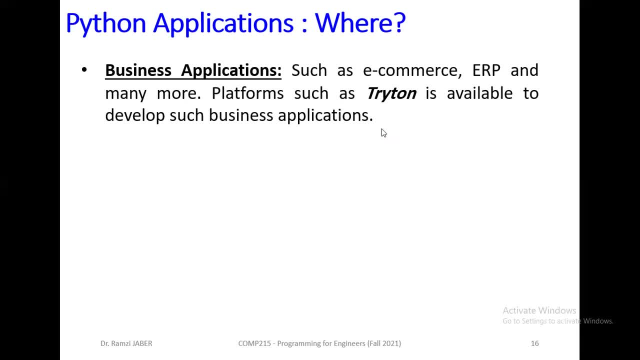 amazon.com alibaba.com and so on they use inside python of course you can use it also in audio and video applications 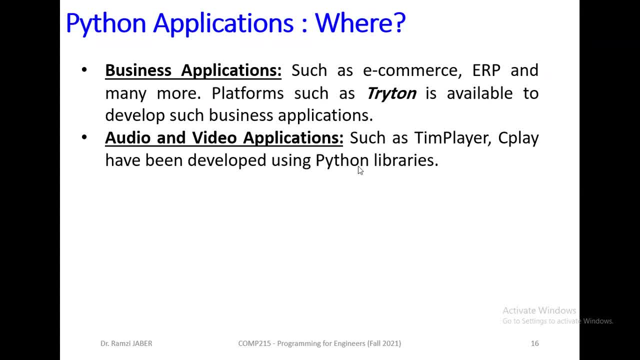 such as time play software c play python using python 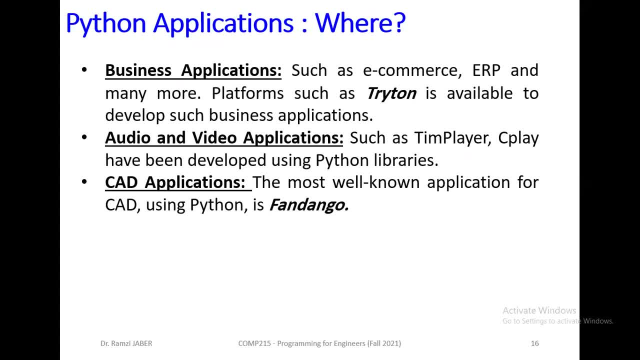 also we can use cad application cad you know cad drawing inside the computer like fandago 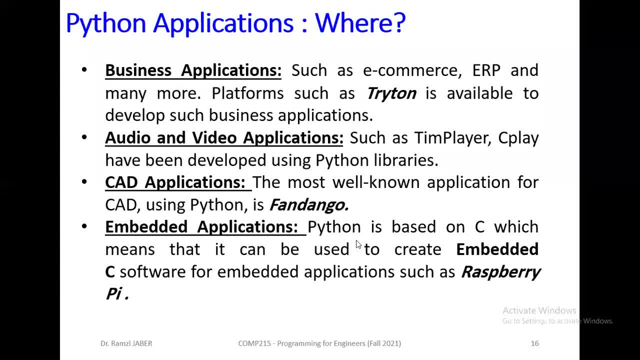 also we can use python an embedded application embedded system 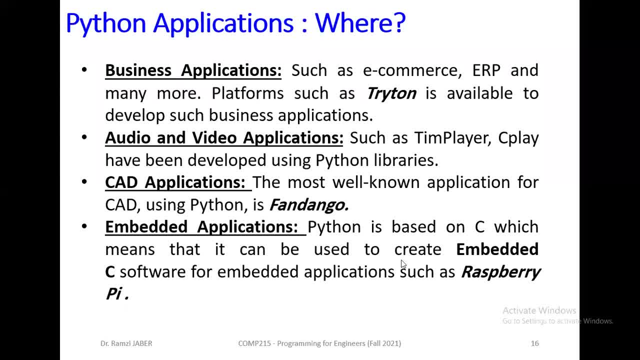 because python is based on c which means that it can be used to create embedded c software so say for an empty system it is a custom file or transfering part of it to another voice so we can use it for embedded applications such as rust presence pi so raspberry pi using python for embedded application or embedded system okay all these we can use python 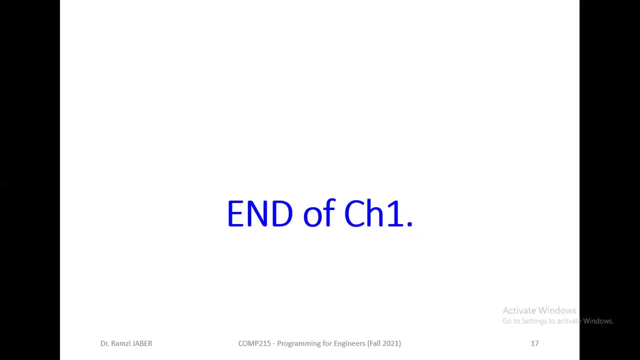 okay so we can use python and everywhere everything okay so Okay, any question on that? 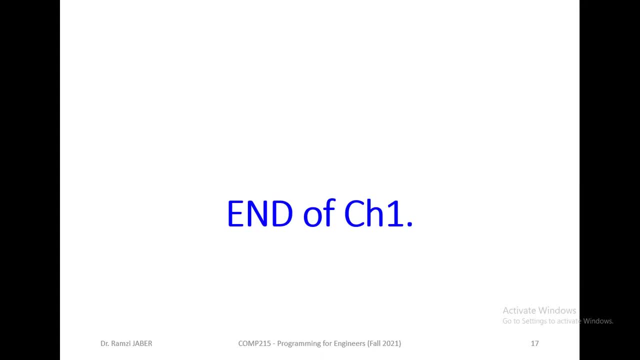 Doctor, which application is used the most for Python? Depends on what you want. Depends on where you're going. What do you want? 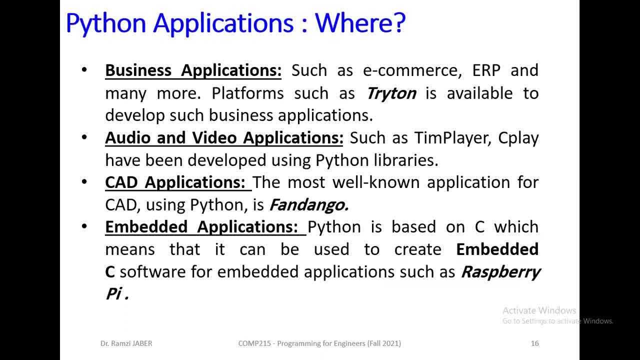 Python is used in all fields. Python can be used in all fields. Like C, like C++, like Java, like other, like other, like functional, like list, like prologue, or other, other. It can even be used like ASP.NET or PHP. It can be used in JavaScript. We can use Python to make code in JavaScript. Okay? So, like JavaScript in the web, web application.